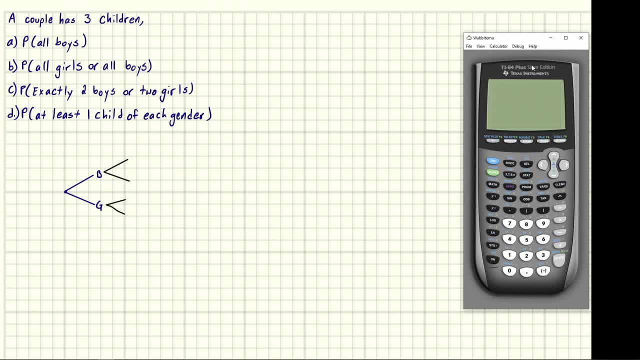 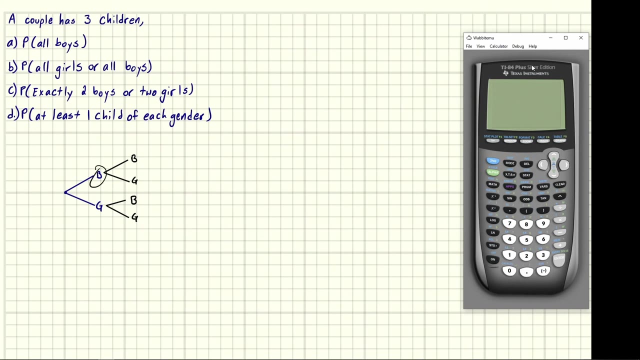 second kid. So here's your second kid. So, given that the first kid was a boy, well, the next kid it could be a boy or a girl. So it's a boy or a girl, and then this could also be a boy or a girl. It's not influenced by the fact that the 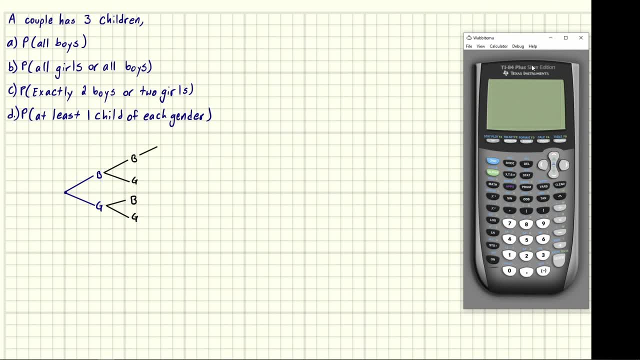 first child was a boy. and then we do it again. We, after our second kid, we have a third kid. So this is the first kid, this is the second kid and here we're going to get the third child. So there's going to be a boy or a girl, and then we do it again after our second kid. 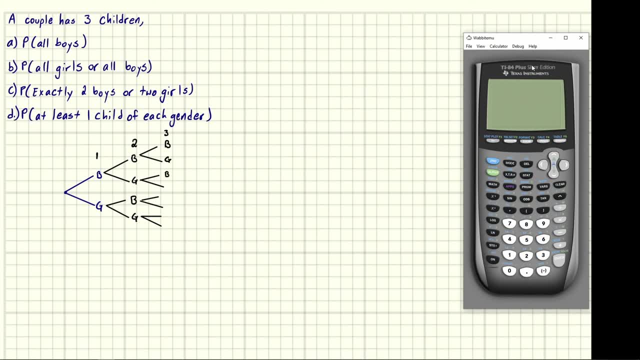 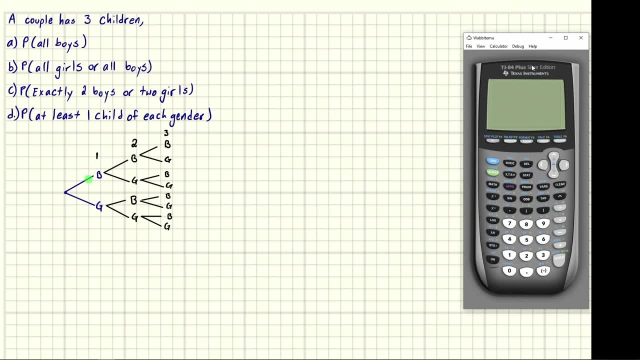 possible outcomes. that could happen, right? So the first child could be a boy, and then we could have another boy and then we could have another boy. right, It could be all boys. or we could have a boy, another boy and then a girl, or we could have a boy, a girl and then a boy. So this, this by 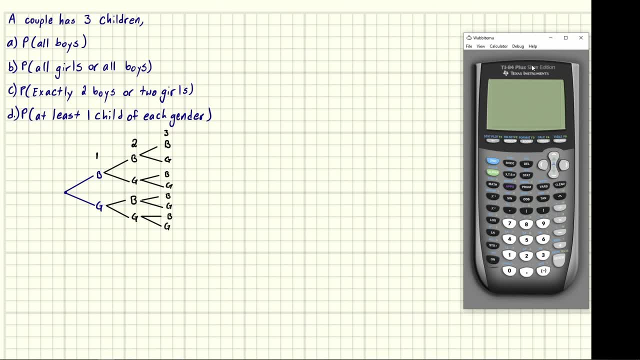 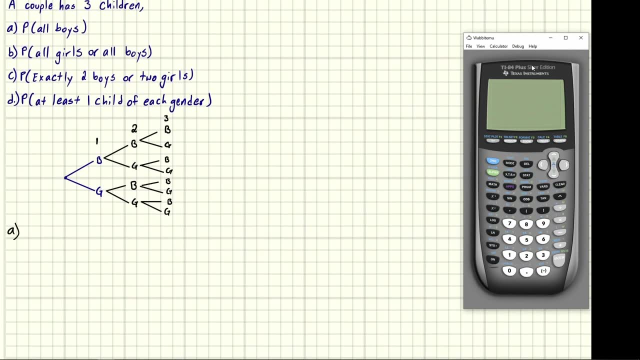 tracing out a path on this, we can find all the possible ways to have three children. So let's go ahead and now tackle part a. and now part a- right are is a probability. So remember probability. we always have our sample space and then we have a condition on top and in this case, our condition. 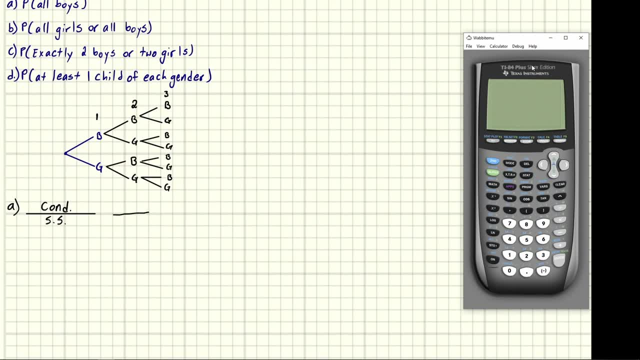 is all boys, and so let's look at that. what is the one path that has all boys? Well, it's right here. boy, boy, boy. there's no other path that has boy, boy boy. all the other paths have a girl somewhere in there. So the chance that you have all boys. well, there's only one of the possible paths that do. 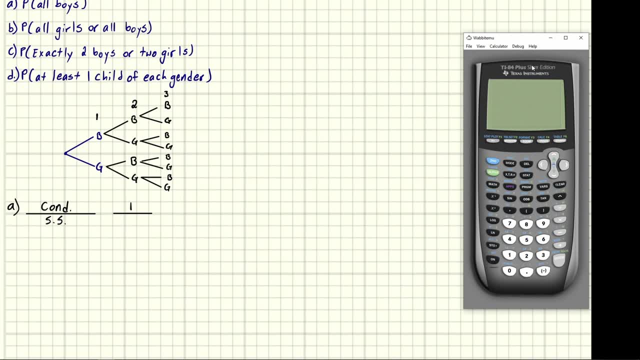 that What's our sample space? well, that our sample space is all the possible paths, and so here, at the very end, all our paths end. So we can just count these. so there's one, two, three, four, five, six, seven, eight possible paths. So there's eight, there's a one eighth chance. you get all boys and I should say: 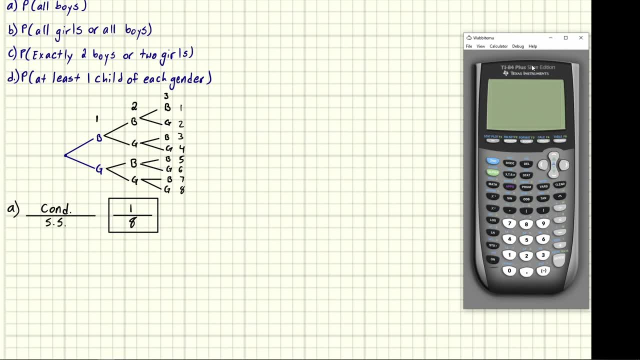 here. there's another way to do this. If you consider the children, here's your first child. this spot is your first child spot. You could have a boy or girl. that's two possible outcomes, and then we're going to multiply that by our second spot. This is our second spot, and then we're going to 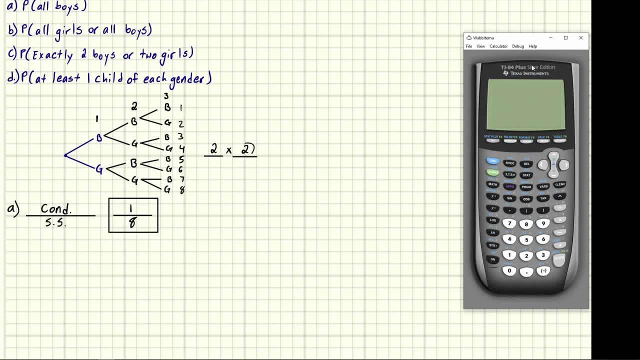 multiply that by our second child, this line, and we could have two possible outcomes, a boy or girl. and then for our third spot, we have two possible outcomes. and look at this two times. two times two, that's eight and that's another way of deducing the sample space. It's because this two is the 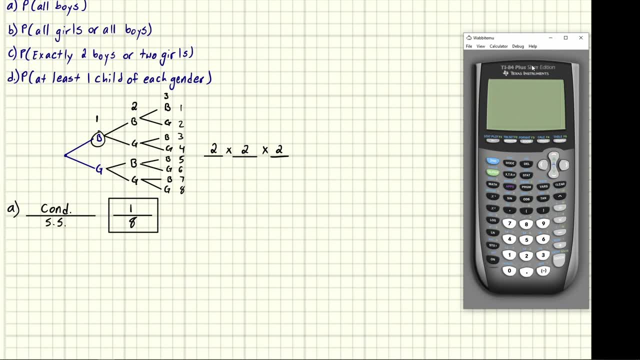 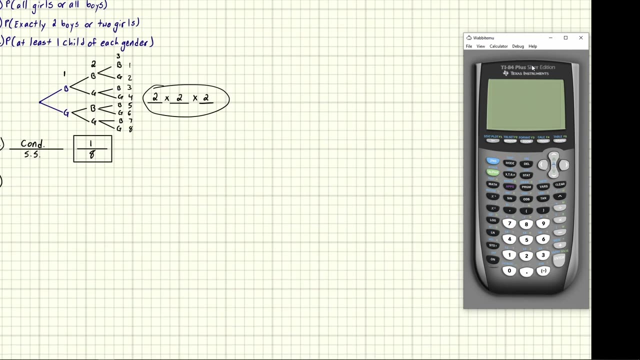 number of branches, from every, from every spot. so like, see, here's a spot and we branched into two pieces and every single spot does this: Here's a spot branched into two pieces. it's the same thing is multiplying and how we can find our total number. So that's A, Let's go to B. So B says: 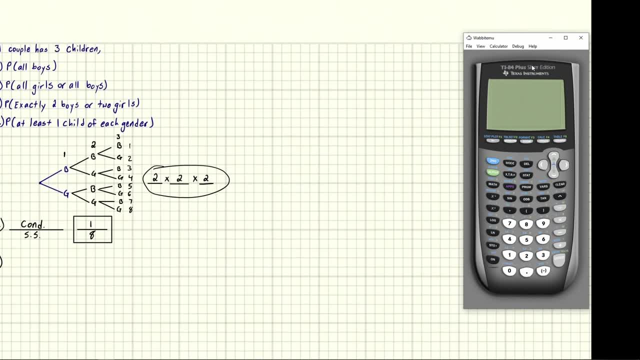 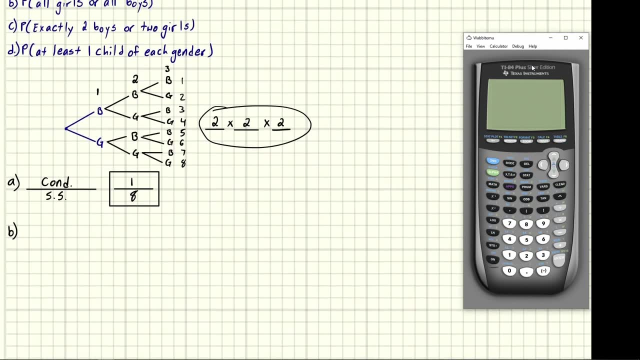 all. oh, it's kind of off the screen here. B says all girls or all boys. So we say, okay, all girls or all boys. Well, the all boys route- we already found that's this right here. And so the all girls routes: girl, girl, girls, right here. all the others have a boy or a girl. 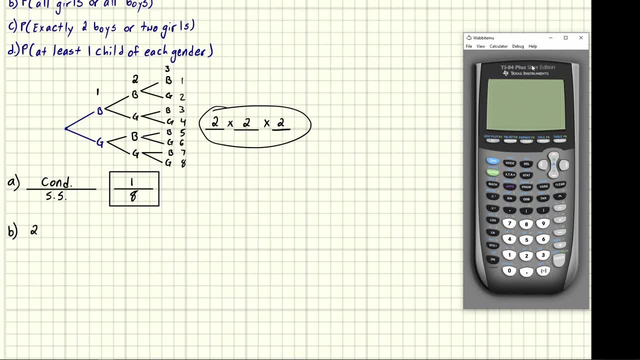 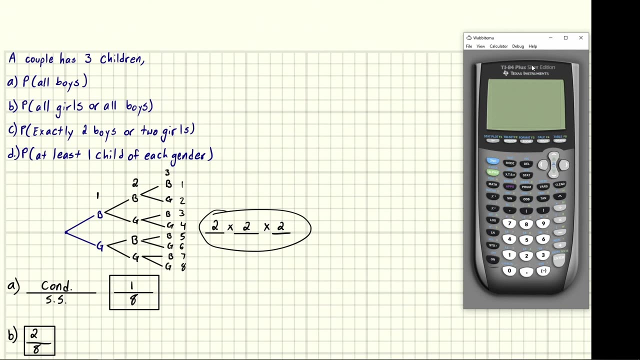 somewhere. So that's two possible routes. So it's going to be two over our sample space, which is eight. So that's pretty straightforward. Now we're going to go for C. C says exactly two boys or two girls, Okay, So at this point it may behoove us to write these: 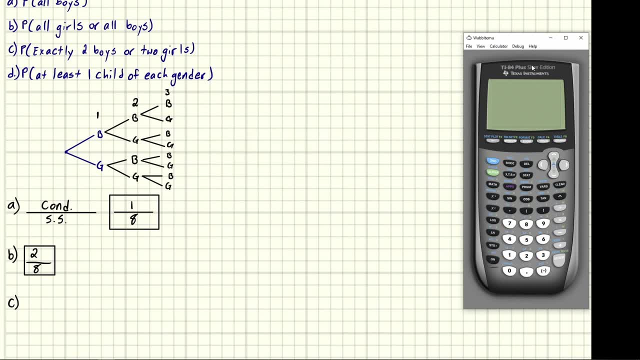 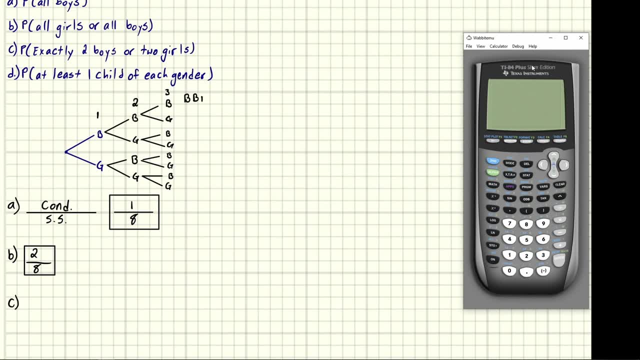 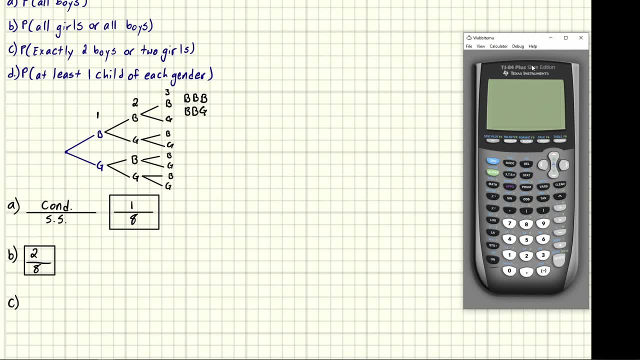 boy girl. we've got boy girl boy, so boy girl boy. and then we've got boy girl, girl boy, girl girl. that's all the ones we can do for this top one. then we've got girl boy boy, so we've got girl boy boy, girl boy girl, girl boy girl. and 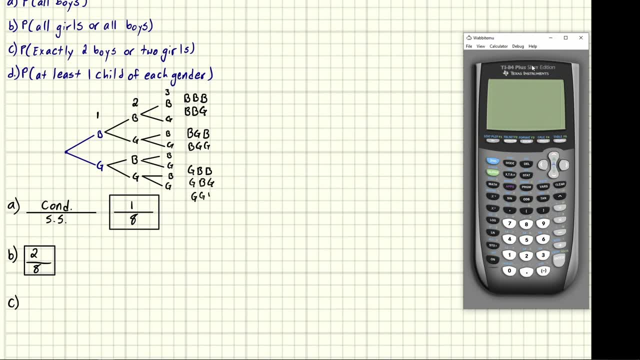 then girl girl boy, girl girl boy and girl girl girl. and just to make sure we didn't miss any, we just count how many we have right. so we should have eight. we have one, two, three, four, five, six, seven, eight. so we got them all and all of. 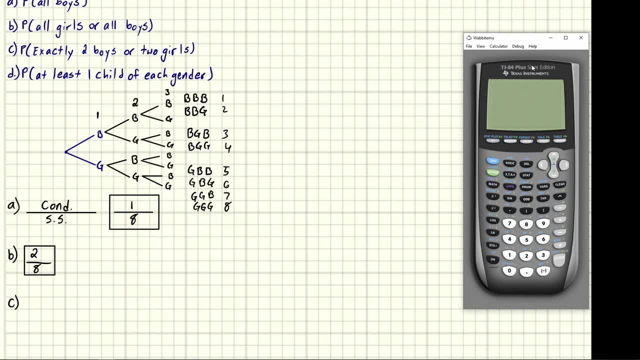 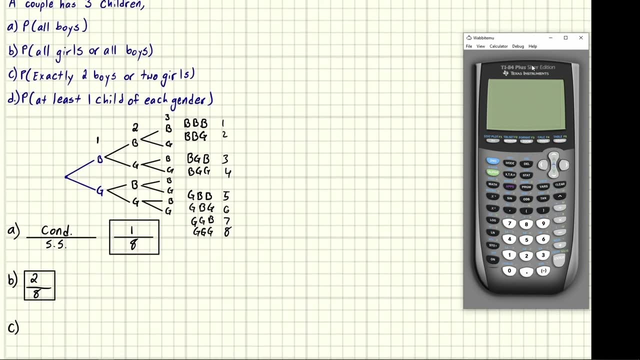 these should be used unique, you shouldn't have any repeating. if you have something repeating, you made a mistake somewhere. so definitely check that we can't have any repeats. and so see, wanted exactly two boys or two girls, and so we just do the ones that have two. 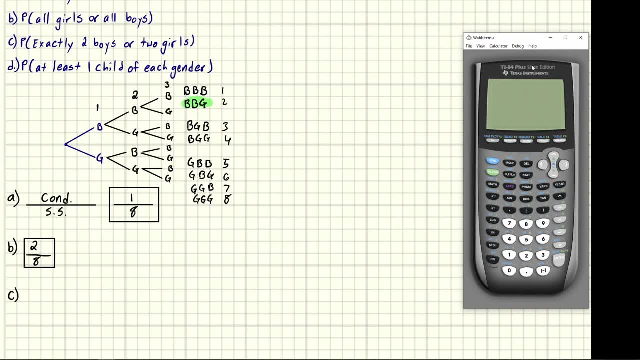 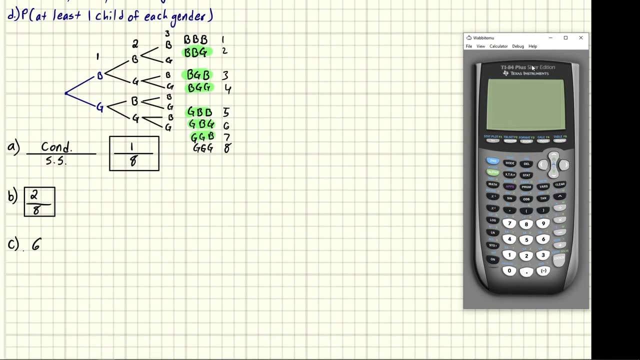 boys or two girls. so here we've got two boys. so there's one, two boys, two girls, two boys, two girls, two girls, and then down here at three girls and three boys. so that won't work. so here we've got six scenarios where, out of the total eight, where we have exactly two boys or exactly two girls. so 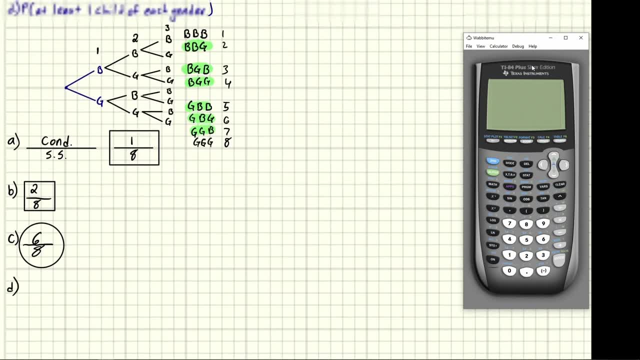 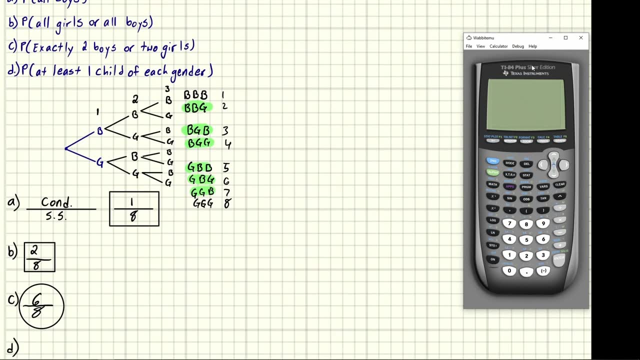 that. see all circle that one, what the heck will be daring. now for Part D: at least one child of each gender. ok, well, at least one child of each gender was think about. that. at least means that there's gotta be a girl and a boy in in the combination, right? because 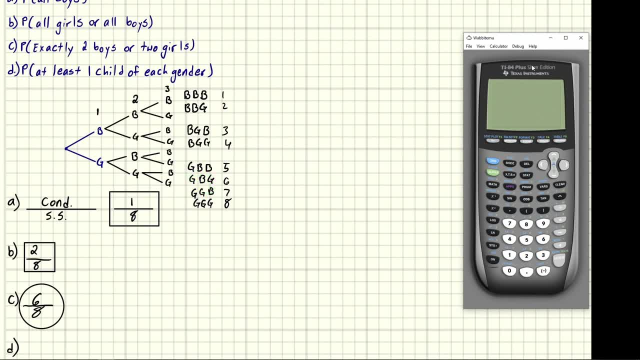 if we have all girls, then we don't have at least one boy, because we need at least one child of each gender. so we need at least one boy and at least one girl, and that will satisfy both the genders. the third child can be a boy or